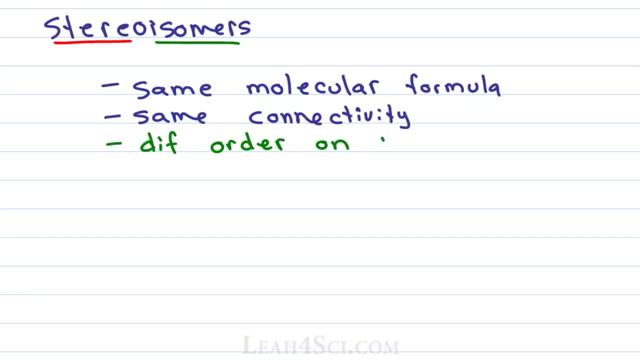 isomers over a double bond or a ring, or stereoisomers, which I think of as chiral isomers, RNFs. When I think of chirality, I think of handedness for the molecule. Many people are right-handed, some people are left-handed, and different tools and machines are meant to be operated. 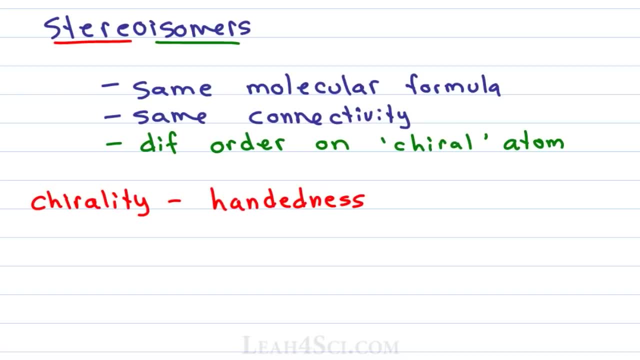 with one hand or the other, the right or the left hand. Imagine taking one of those big, heavy fancy gloves that's meant for your right hand and putting it on to your left hand. it just doesn't work. Right now we're going to talk about the structure of chirality. We're going to talk about the 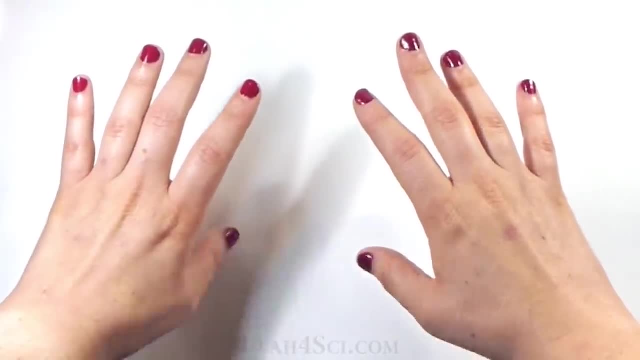 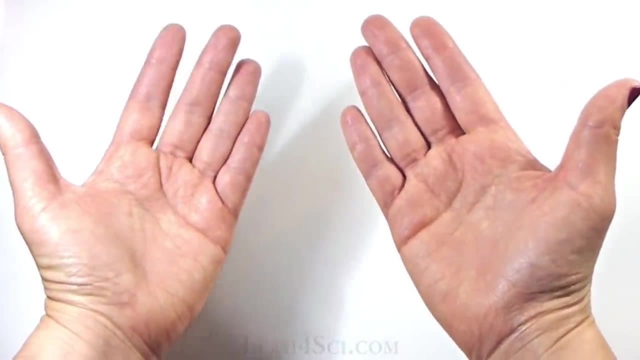 structure of chirality. Right now, we're looking at the top of my right and left hand, and they look about the same. I have thumbs in the same place, fingers in the same place, and when I turn it over, they still look the same. So, while hands are the same, though, notice that no matter how, 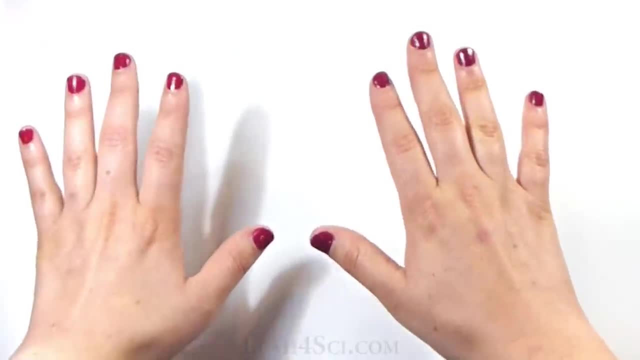 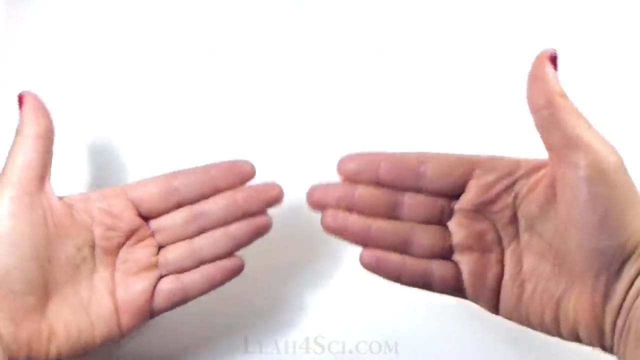 I turn them, imagine there's a mirror right here between them. Right now, my thumbs are mirrored, fingers are mirrored. there's still an imaginary mirror between them, still an imaginary mirror. No matter how I turn them, it appears that there's an imaginary mirror. 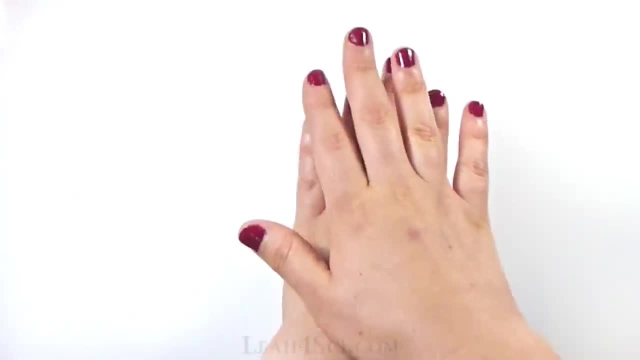 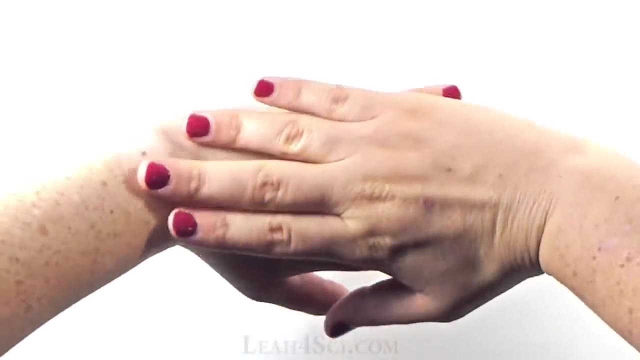 between them. But now what happens if I try to superimpose them? Well, my thumbs are sticking out. So if I turn it now, my fingers are in opposite direction. If I flip my hand so that my thumbs and fingers are aligned, well, my palms are in opposite. 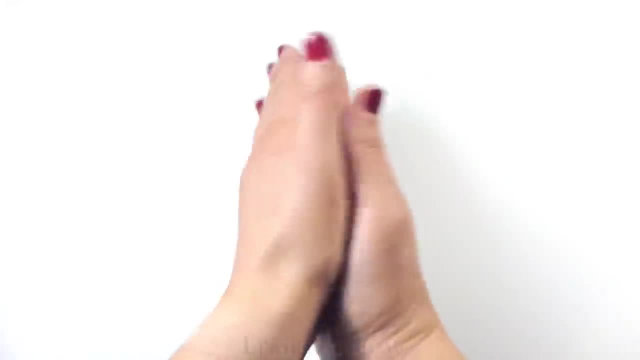 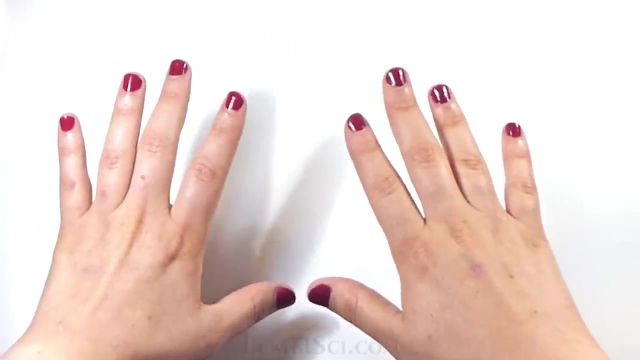 direction. No matter what I do, there's no way for me to perfectly superimpose my right and left hand, making them mirror images to each other. So we agree that hands are mirror images to each other, and if these are your right and 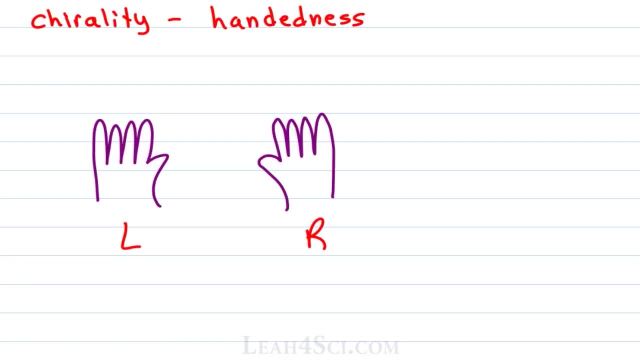 left hands. palm down is the right hand. Okay, Okay, Okay, Okay, Okay, Okay, Okay, down on the table. they are the same, but they're mirror images of each other, And the only way that you can superimpose a hand would be if you took a thumb and added it to the 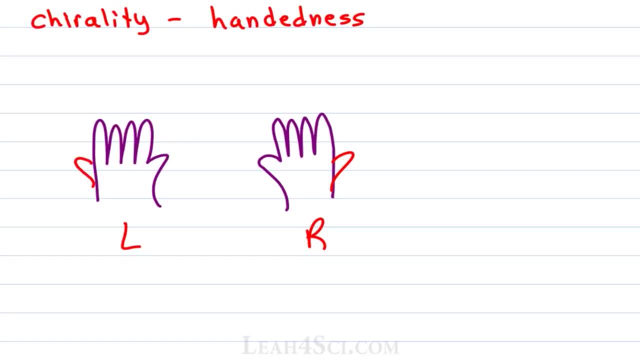 other side, assuming the fingers were the same- took a thumb and added it to the other side. Now you see, the right and left hand are exactly the same. In fact, there is a plane of symmetry going right down the middle, and that is the key. If there is symmetry, then your two hands. 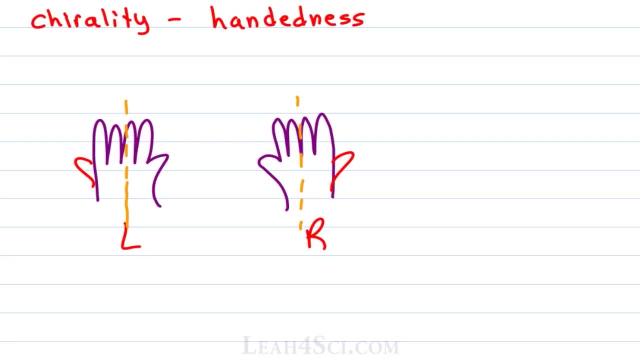 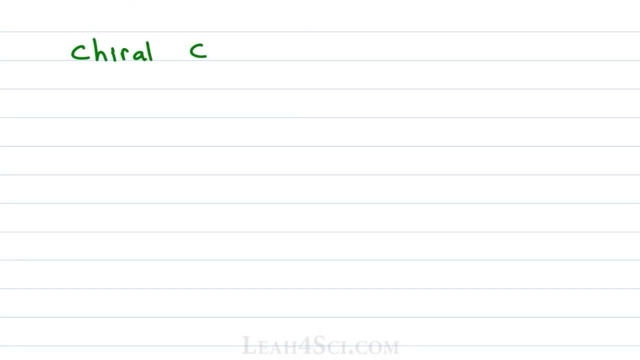 will be superimposable and they will not be unique. A right two thumb glove will fit a left two thumb hand, and the other way around. When thinking of chirality, we're typically looking at a chiral carbon. Every now and then you'll see a molecule that is chiral. 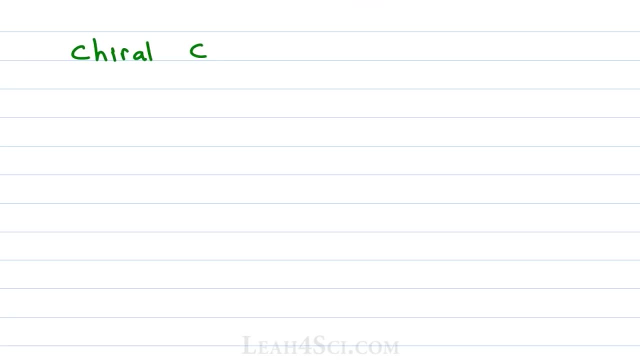 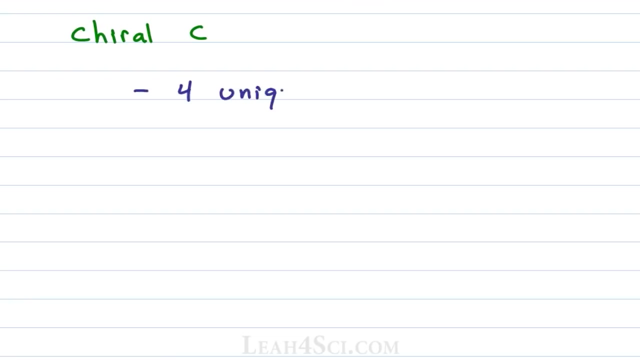 as a whole, or a nitrogen, for example, with four substituents and a positive charge, 99% of the time it'll be a chiral carbon. A chiral carbon must have four unique substituents. If they're not unique, it's like a chiral carbon. 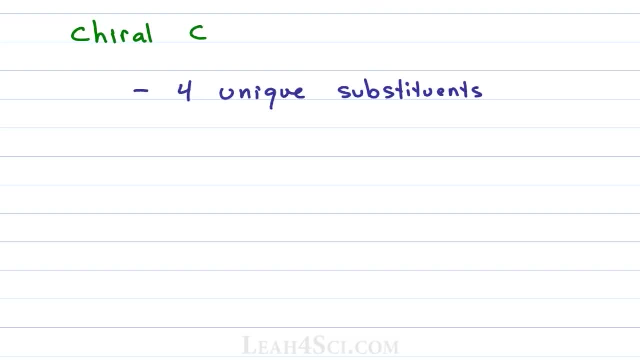 It's like having a two thumb hand, and they'll be superimposable. In order to have four unique substituents, we're looking at four bonds to carbon, and that means it must be sp3, hybridized and tetrahedral in its shape. 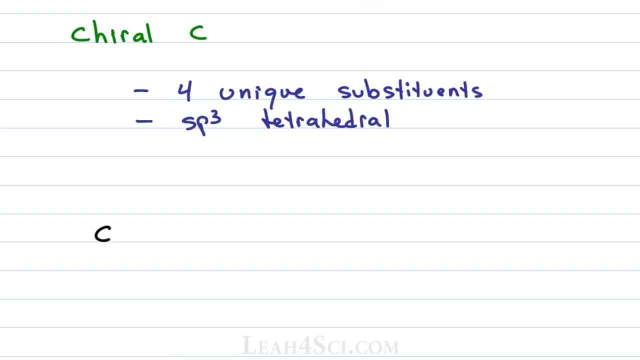 So, for example, if I show you a carbon here and I draw it in three dimensions so that I have two bonds in the plane of the page, one up, one down to the left, I have one coming out down but out of the page and one down and into the page. This is just one of the 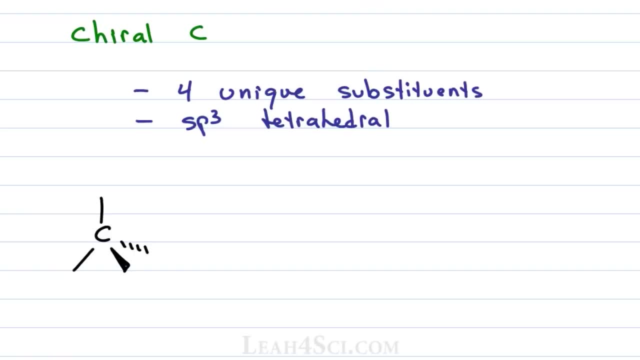 methods that you can use To draw a chiral molecule, but the key here is to recognize. we have four substituents and so they'll have to be unique. We'll show A, B, C and D. I'm using these colors so that 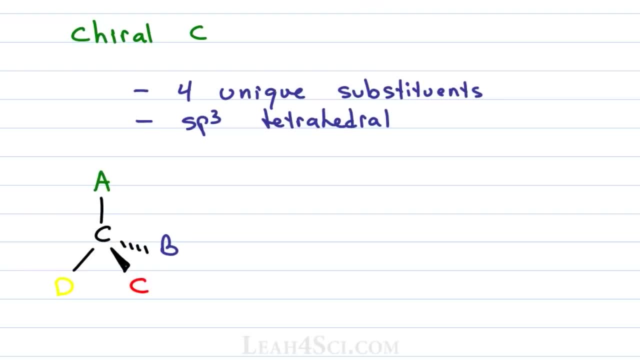 we can follow along with a model kit where the yellow represents the white. Four unique substituents on an sp3. hybridized tetrahedral carbon gives me a chiral carbon in the center. This central or chiral carbon is referred to as the stereocenter. 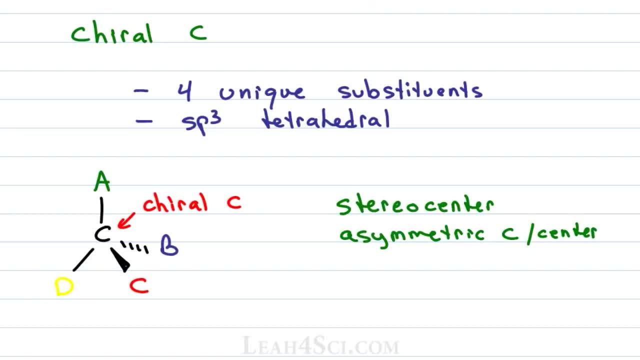 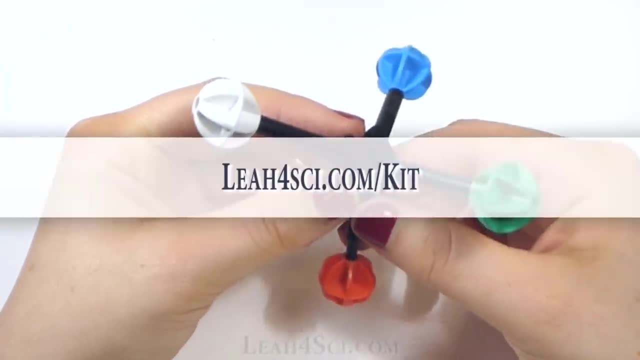 Or the asymmetric carbon or asymmetric center In organic chemistry. it helps to look and hold the 3D structure. If you don't have a kit yet, get one on Amazon by going through leah4scicom slash kit and if you purchase, 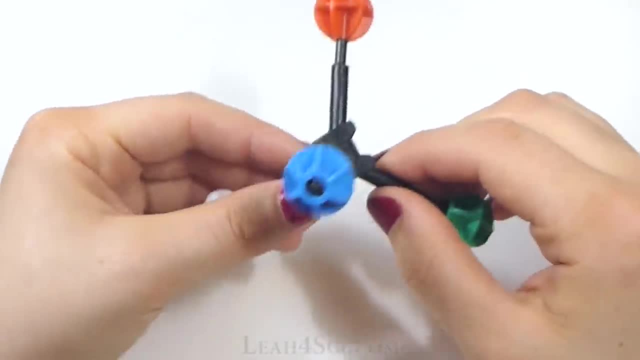 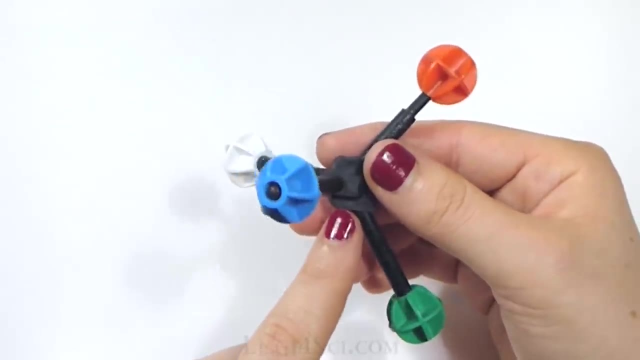 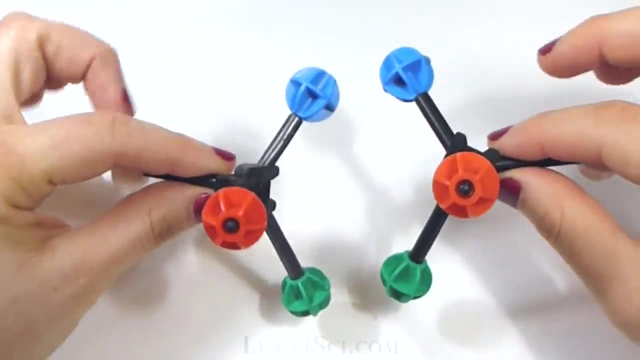 through my link, I do get a small commission. So notice, here we have a central carbon atom with four unique substituents. This is considered the chiral or asymmetric center, and it's tetrahedral because it's sp3 hybridized. So notice that I have two apparently same looking structures where each one has a chiral. 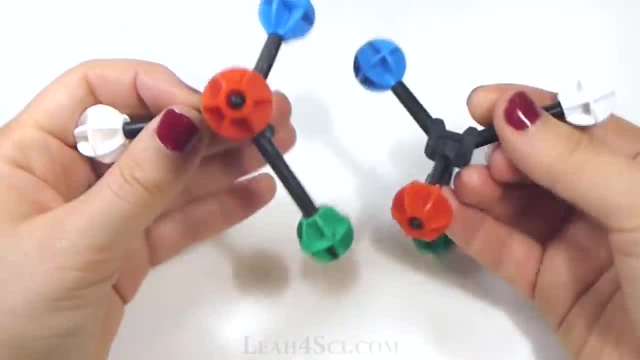 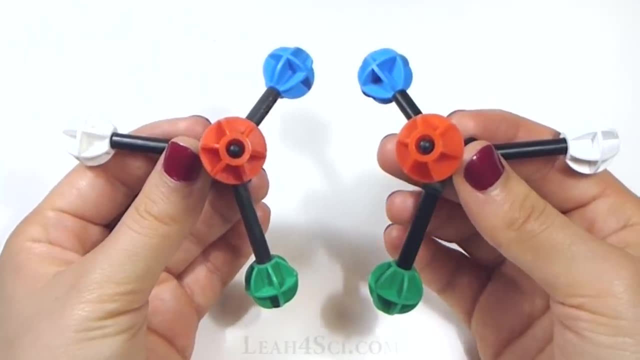 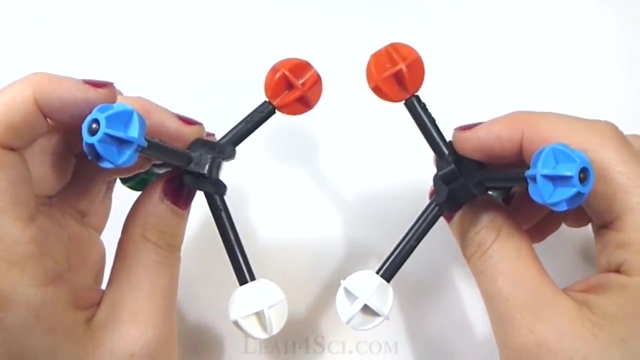 center and the four same substituents. If you look at the two molecules, you can see an imaginary mirror between them, because they are perfectly reflected in each other. And as I turn them, they are still perfectly reflected in each other, Since these are chiral with an sp3- central carbon and four unique substituents. because 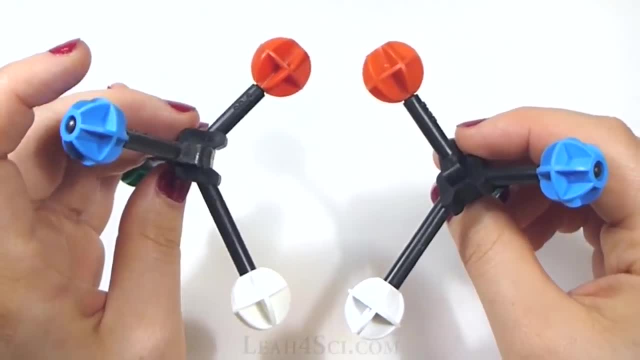 they have a mirror, they are still perfectly reflected in each other, Since these are chiral with an sp3, central carbon and four unique substituents. because they have a mirror between them, they are considered enantiomers or mirror images And no matter how I turn. 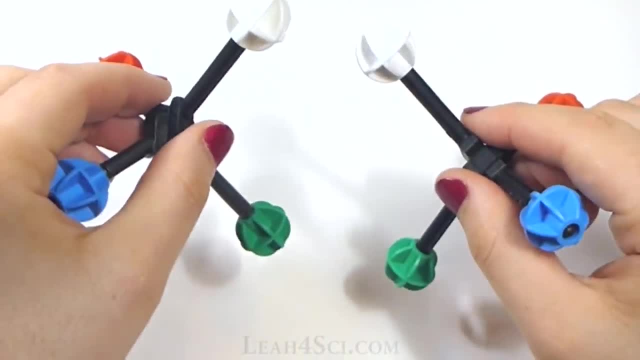 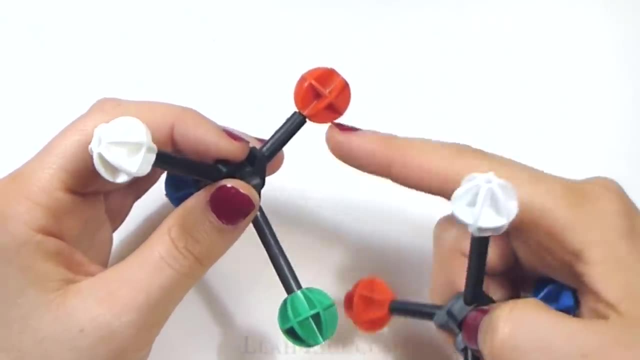 them. I can always find that mirror between them. But now, if I try to superimpose them, let's see what happens. To place one on top of the other, I need these substituents to line up. So let's flip it and line up the red and the green. But look at what happened. 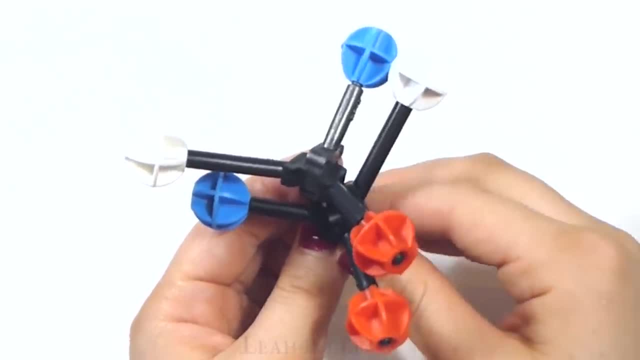 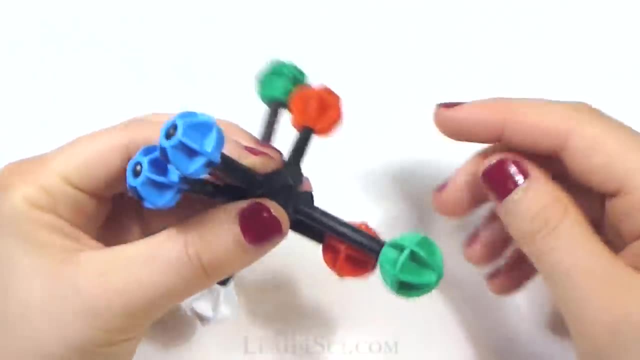 The blue and white do not line up. If I try to switch it so the blue and white are lined up, then look what happened to the red and green. They don't work. They don't work, They don't match. Just like, with my hands, something is sticking out- Remember it was thumbs or 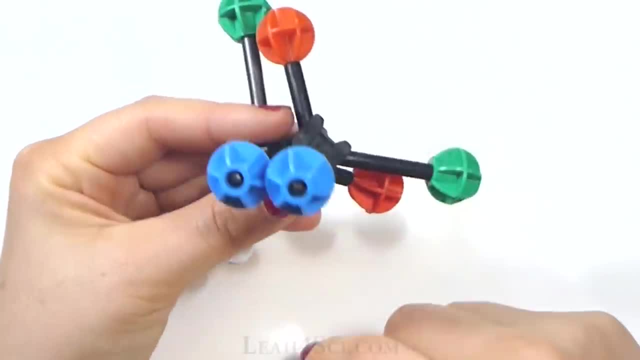 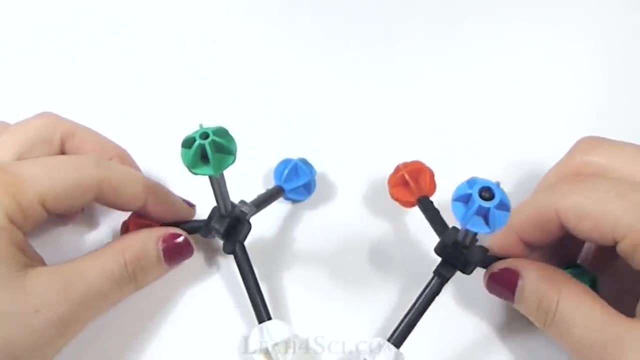 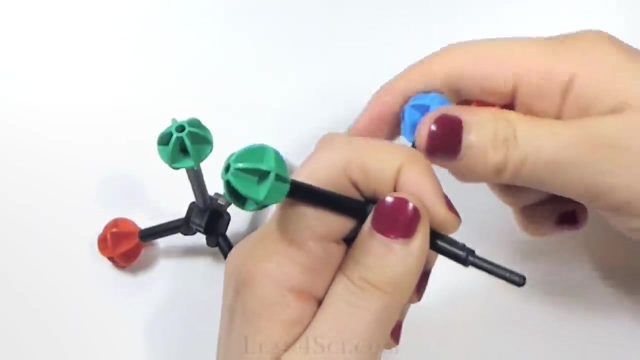 fingers Here. the only way to line up two of the substituents is to have the two other substituents be opposite. In fact, the only way I can superimpose these two is if I take some of the bonds and physically break them, moving the substituents around just like. 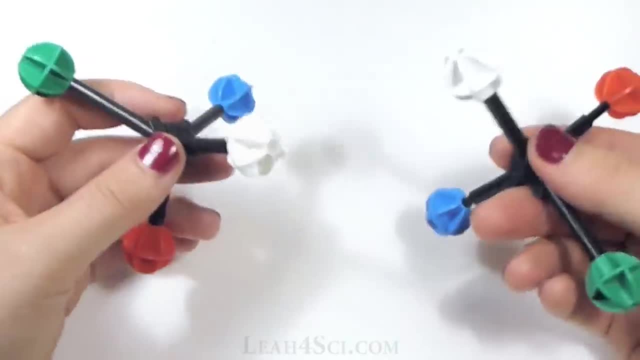 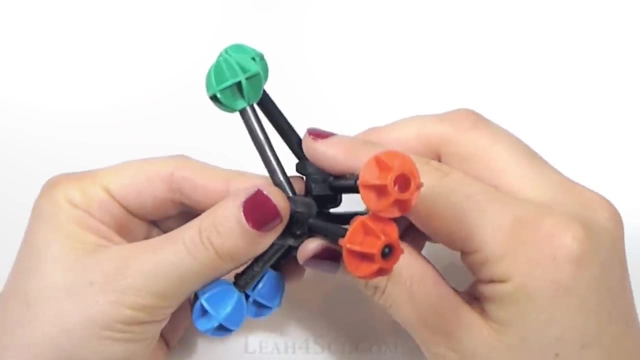 the example of moving a thumb to the other side. And now look what happens. The blue is lined up, white, green and red. they are perfectly lined up. They're still chiral, but now they're two of the same chiral molecules rather than mirror. 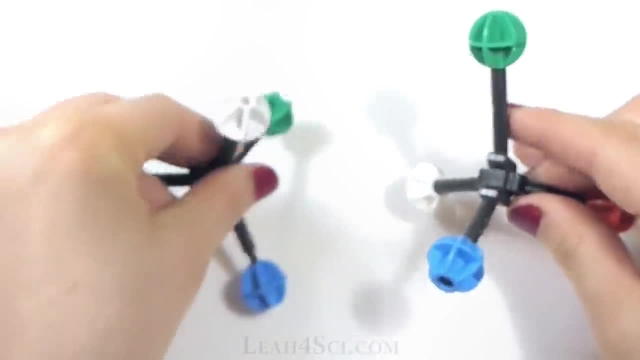 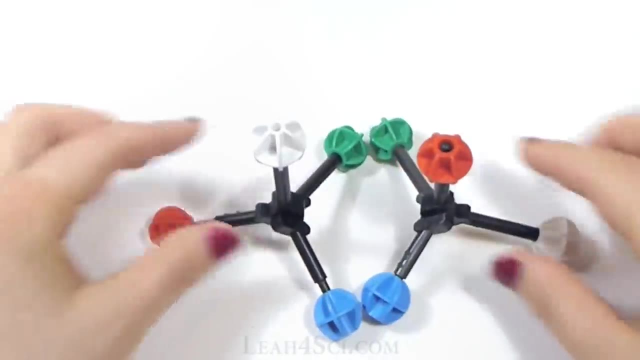 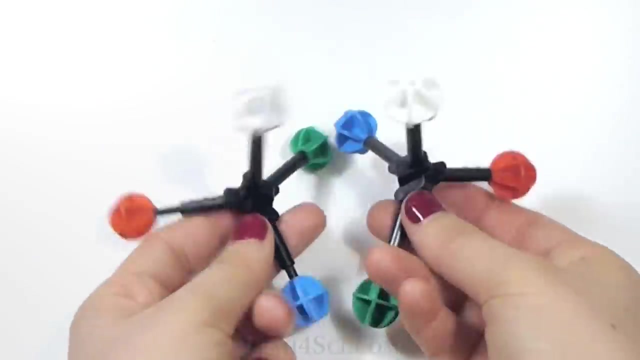 images of each other. Let's prove it by trying to reflect them in each other. Look at that. The green and blue are reflected, but the red and white are opposite. They don't line up. If I try to put a mirror between the red and white now, the blue and green don't line up. 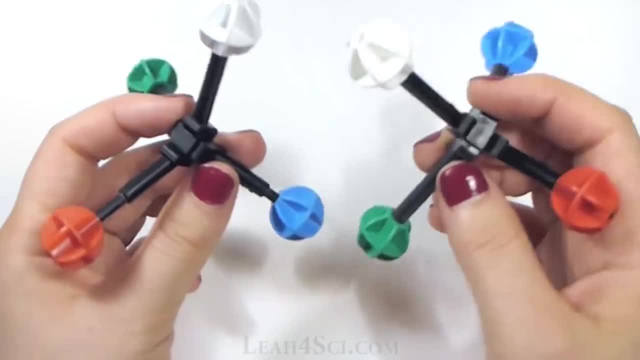 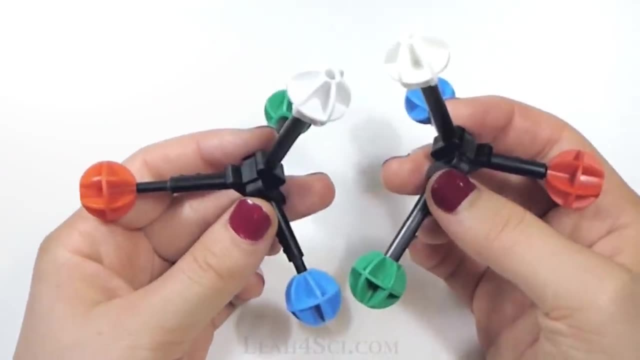 So, no matter what I do, I will not be able to show these as mirror images, because if they're chiral and they're the same, they're not enantiomers of each other, right? They're either the same or enantiomers. 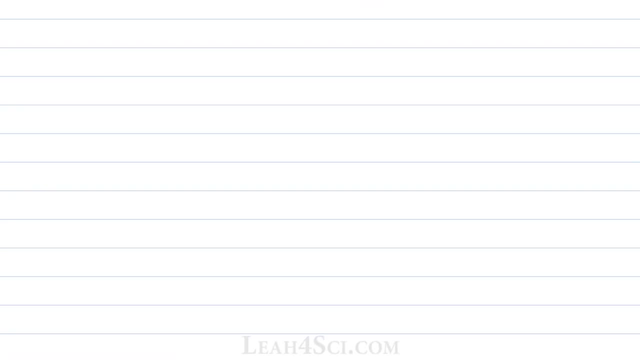 So we have the option for two different types of molecules when it's chiral. Going back to the hand example, if you have a right hand and a right hand, they're exactly the same. They'll fit the same gloves. They'll be superimposable with each other. We are gonna call them the same If we have. 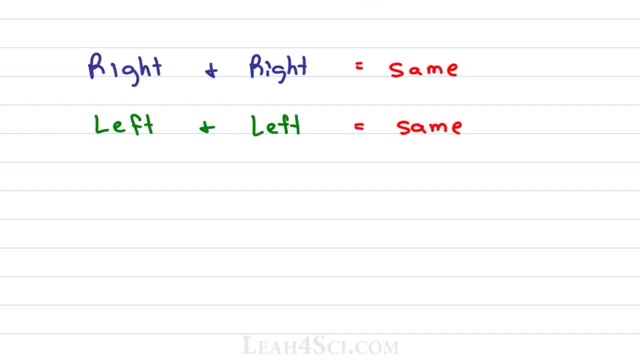 a left hand and a left hand. they're the same, Or we're gonna call the same. So let's see hand once again. they are considered the same. They are superimposable. Superimposable tells you that you can take one right hand and put it on top of the other right hand. 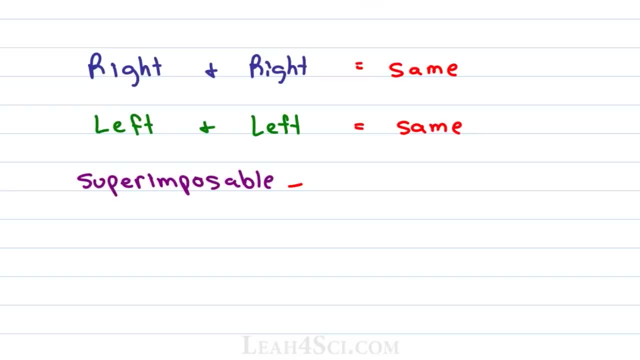 and it'll look exactly the same. or take one chiral molecule and another molecule of the same chirality and put one on top of each other- they look exactly the same. There are two scenarios where you'll see a superimposable molecule If you have two chiral molecules. 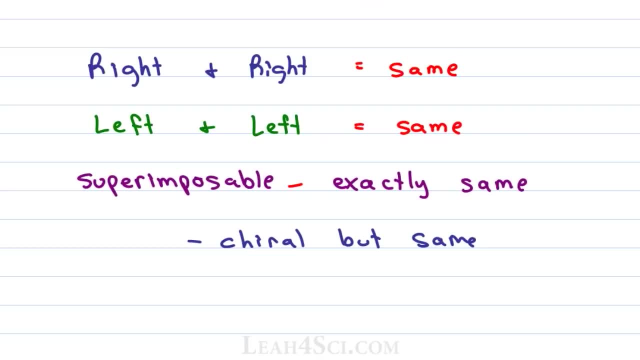 but they're exactly the same meaning. they're not mirror images, they are considered superimposable. or if you have an achiral molecule, a molecule that is not chiral because it has a plane of symmetry. For example, if you have a carbon with three rather than four unique substituents. 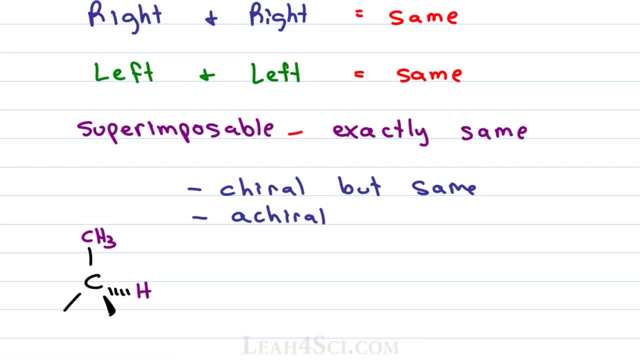 for example, this central carbon has a methyl, a hydrogen, another hydrogen and an OH hydroxy group. In this case, having two hydrogen atoms means this molecule has a plane of symmetry, and if it's not easy to see here, build it on your model kit and rotate it in this direction. 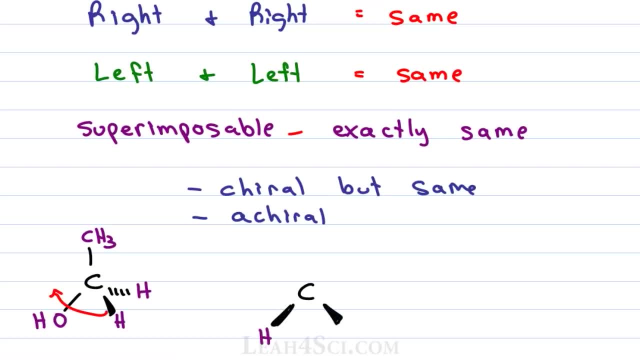 so you have the hydrogens on the right and left. We have two hydrogens coming out of the page, one to the right, one to the left. There's an OH going down and towards the back There's a CH3 going straight up in the plane of the page. and look at that symmetry, right. 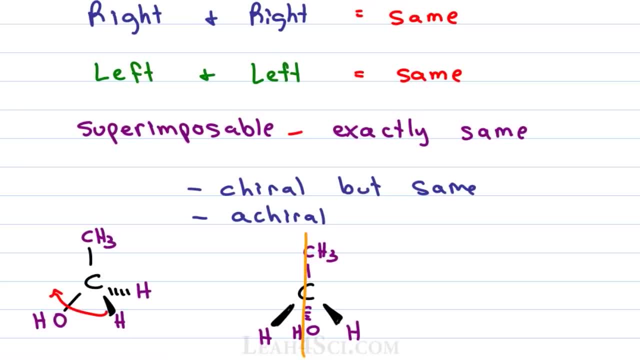 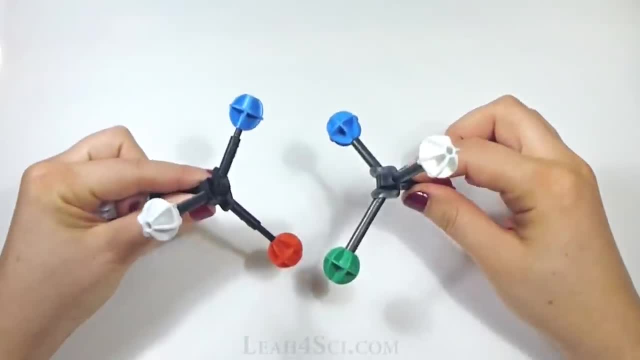 down the middle. So if your molecules are chiral but the same, or if they're achiral with a plane of symmetry, they are going to be superimposable. Now let's see what happens if, instead of four unique substituents, I have only three. So 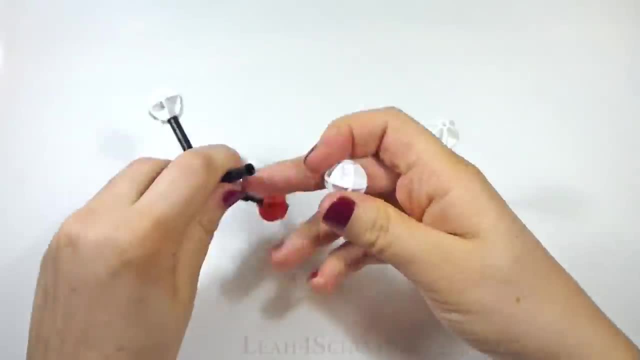 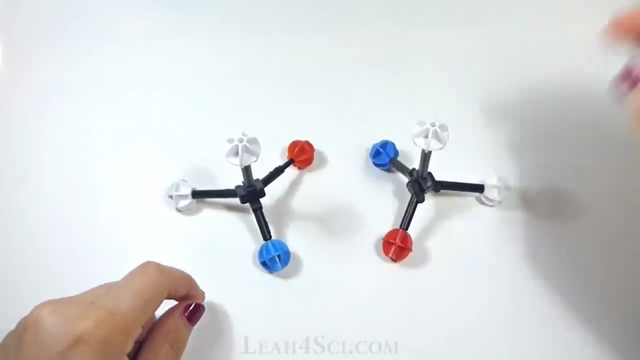 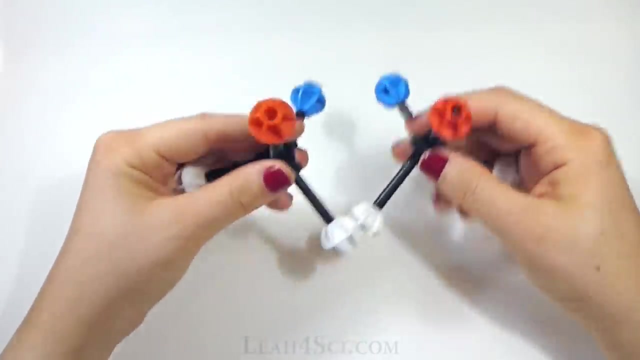 we'll take off the green one and swap it for white. So let's start with creating mirror images. I have the red and blue. Red and blue. they are perfect mirror images of each other. But how is it possible to have mirror images if I can take the same molecule and superimpose? 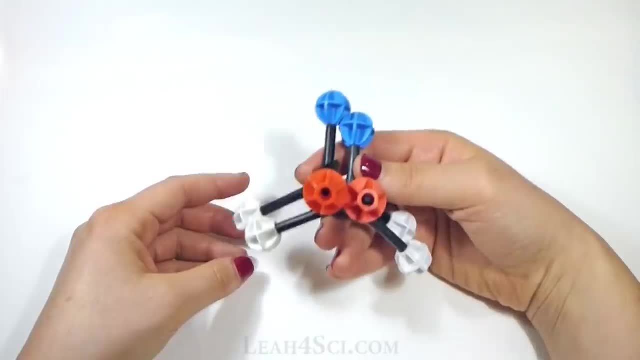 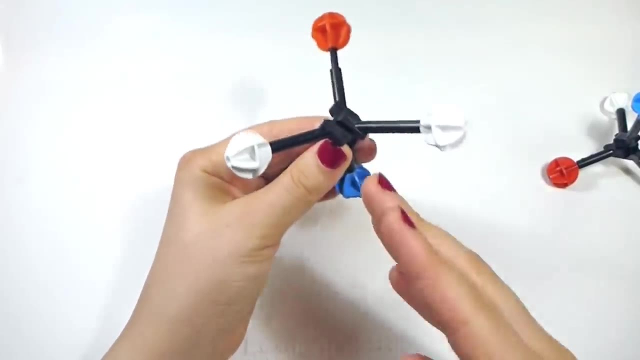 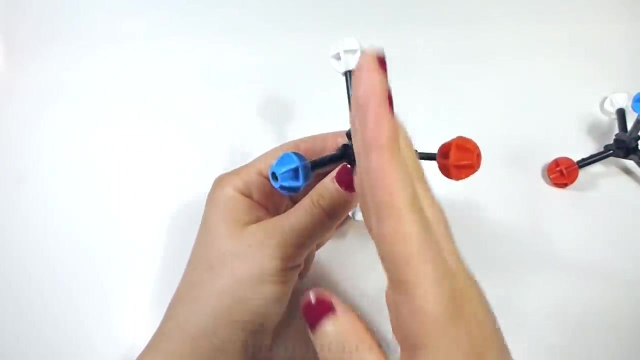 it on the other one. How is a superimposable molecule also a mirror image? And the answer is: two of the same substituents makes this molecule symmetrical. Notice there's a line of symmetry going right down the center- Again a line of symmetry. no matter how I turn it, I can find that symmetry. 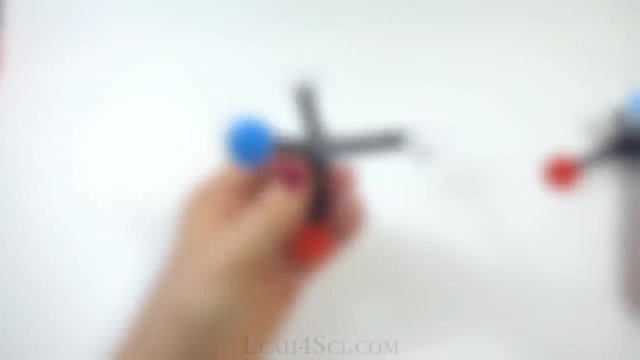 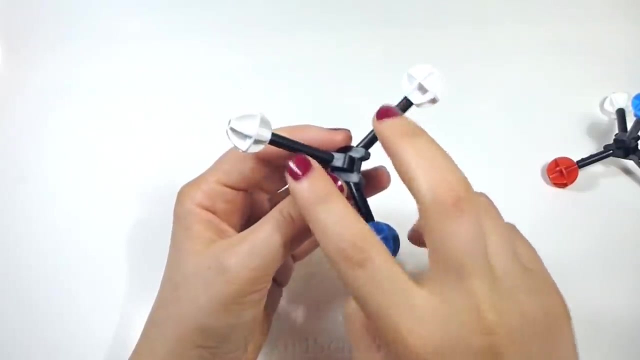 and that makes this molecule achiral. Because this molecule has a tetrahedral sp3 carbon in the center, but two of the same substituent, for a total of three unique substituents. you're unique, it's not chiral. And if it's not chiral it doesn't have a mirror image, it's going. 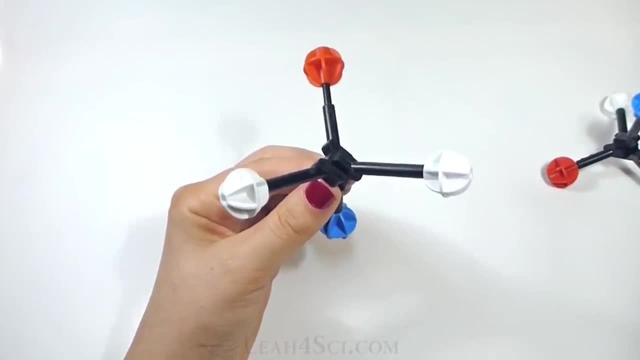 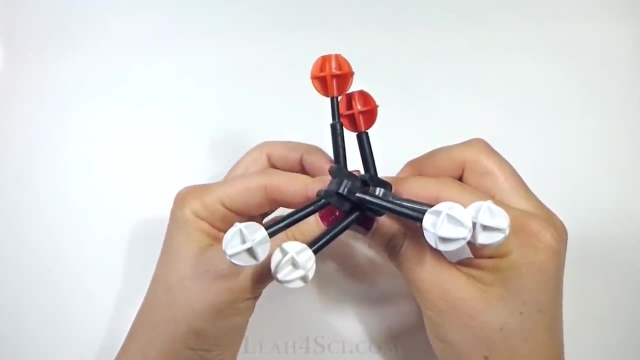 to be superimposable on another molecule of its kind. And just because it's superimposable doesn't make them enantiomers. it just makes them superimposable because they're the same exact thing. If you have two molecules that are chiral but they're opposite chirality. 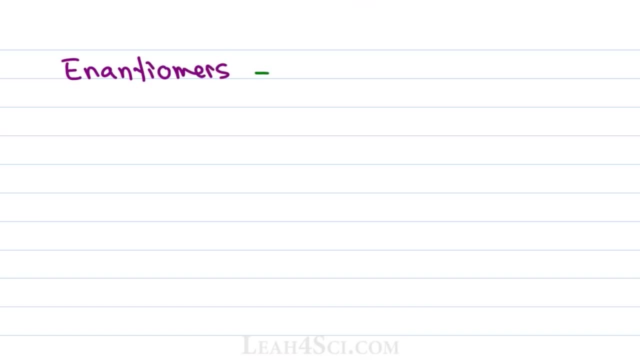 meaning right-handed and left-handed- then they are considered enantiomers. Enantiomers are chiral molecules that are non-superimposable because they're opposite to each other, and another common term you'll hear for this is mirror images, because one reflects into the 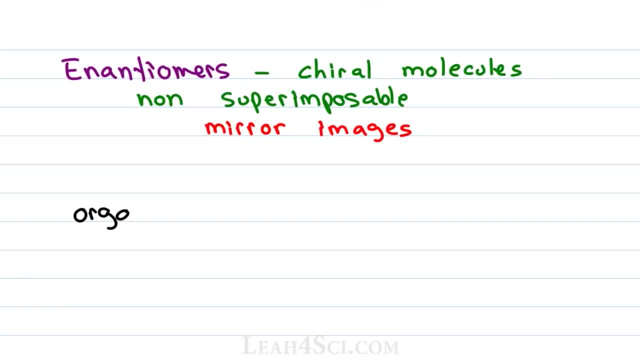 other. In organic chemistry we classify chiral carbons or chiral atoms as being R or S. In biochemistry and sometimes in organic chemistry, when looking at organic molecules, you're going to use the DNL configurations, which tells you how it rotates: plane polarized light. 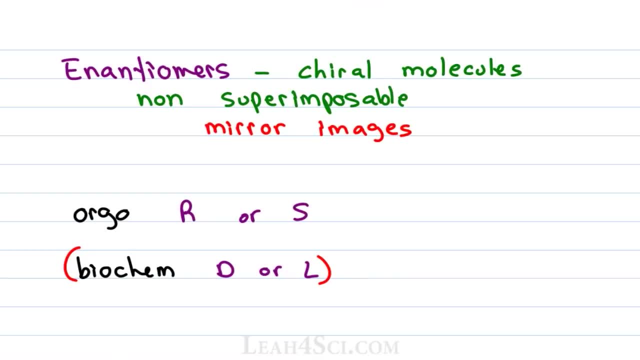 and what. we're not going to discuss it in this video, but we're going to discuss it in this series. Just keep in mind: R and S does not equal to D and L directly, because some R molecules will be D, some R will be L and the other way around. So how do you tell if? 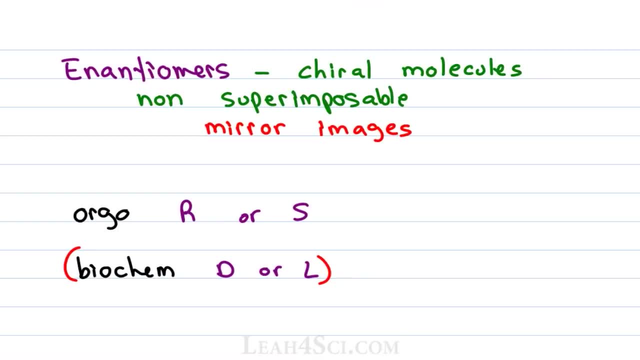 a molecule is R or S in organic chemistry. That's exactly what we're going to discuss in the next video. You can find this entire video series, along with the chirality and stereochemistry practice quiz and cheat sheet, by visiting my website: leah4scicom. slash chirality. 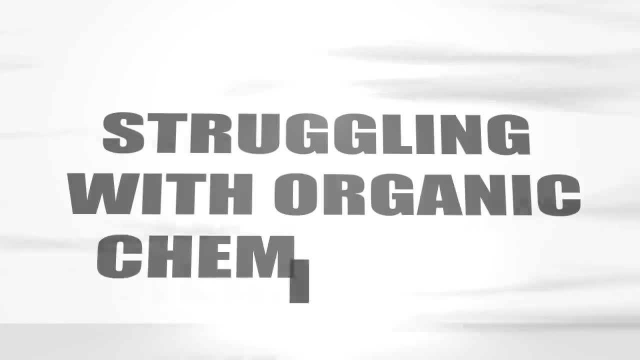 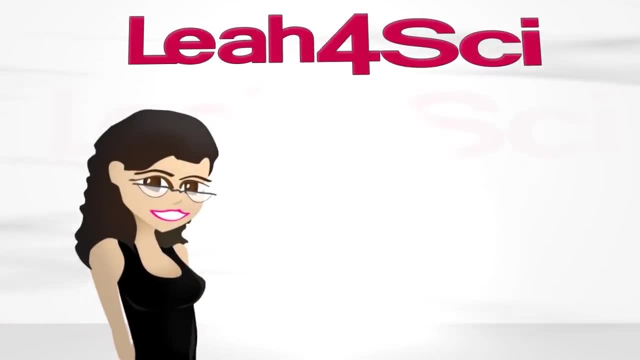 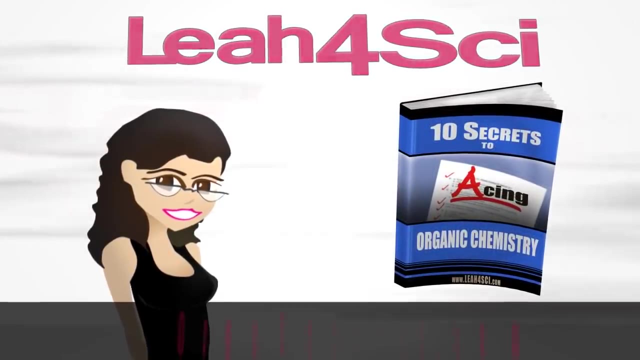 Are you struggling with organic chemistry? Are you looking for resources and information to guide you through the course and help you succeed? If so, then I have a deal for you: A free copy of my ebook 10 Secrets to Acing Organic Chemistry. Use the link below or visit.